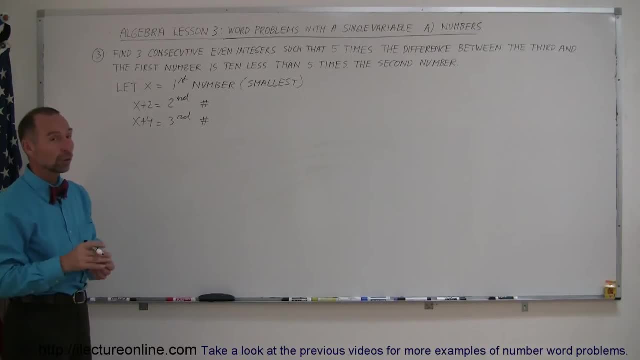 And it says that five times the difference between the third and the first number. So five times the difference Between the third and the first number. So that's the third number minus the first number. So let's see if we got this right. So it's five times the difference between the third number and. 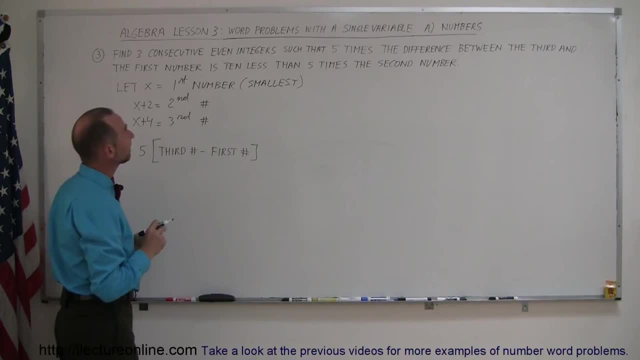 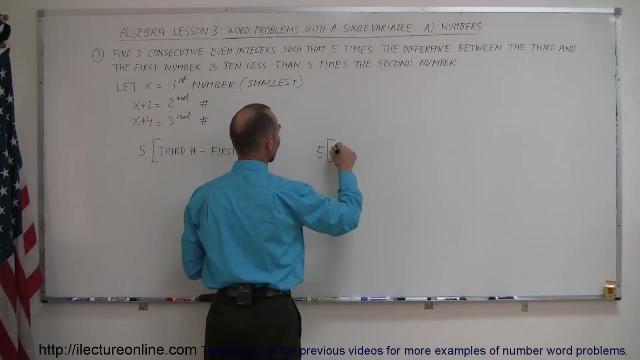 the first number. So we got that right And that should be ten less than five times the second number. So here we have five times the second number And that's equal to: And this is ten less than this. So it's this minus ten, So this is equal to ten less than five times the second number. 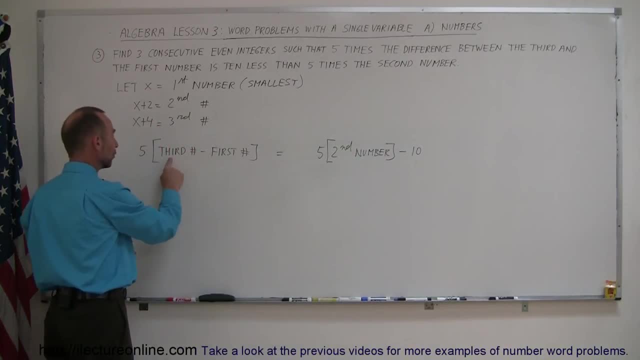 All right, Again, five times. the difference between the third number and the first number equals ten less than five times the second number. Now we can go ahead. what each one of those are equal to The third number is x plus four times X plus 4 minus the first number, which is X, and that is equal to 5 times. 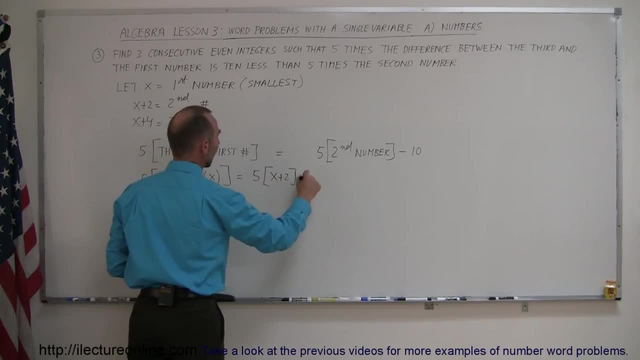 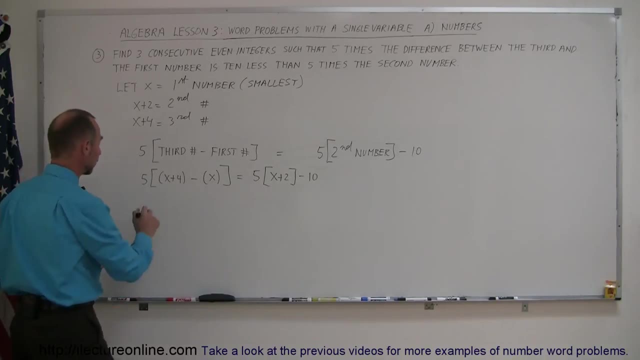 the second number, which is X plus 2 minus 10, and now we can go ahead and solve that equation. solve it for X. so first we want to get rid of the parentheses and the brackets, so we can say that 5 times X plus 4 minus X is: 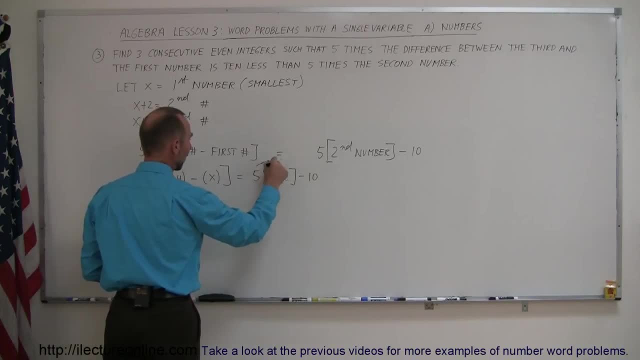 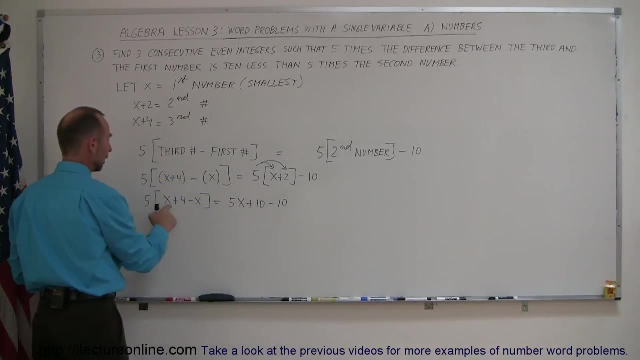 equal to. we can already multiply this out. so 5 times X and 5 times 2, that gives us 5 X plus 10, and then we still have the minus 10 here. then X minus X is simply 0 plus 4. so we have: 5 times 4 is equal to 5 X plus 10 minus 10, and so we 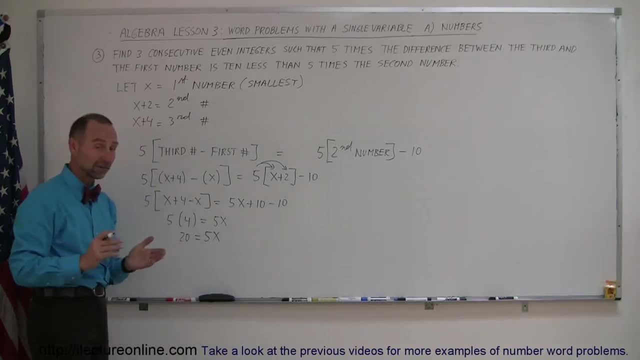 have 20 is equal to 5 X. now, since I'm solving for X, I'm going to turn the equation around, move the 5 X over here and the 20 over there, so we have 5 X equals 20. and now we divide both sides by the coefficient, and so we have X is equal to.